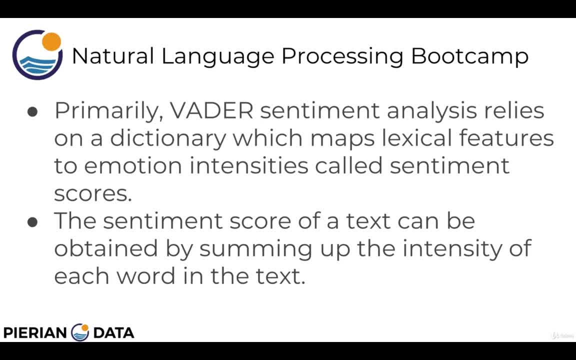 intensities, called sentiment scores. The sentiment score of a text can then be attained by summing up the intensity of each word in the text. We'll talk about that in a little bit, So let's go ahead and take a look at the text. So, essentially, every single word has some sort of positive or negative. 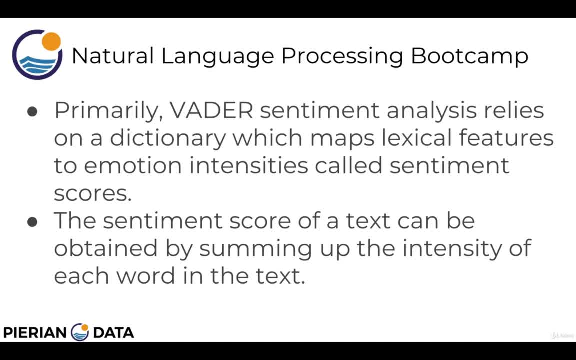 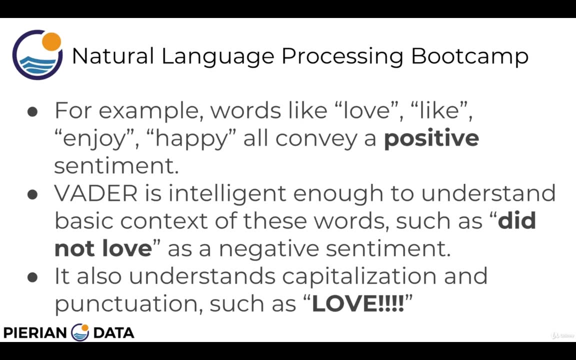 value attached to it. And what we do is we just take all the words inside of a text document and then convert them into positive or negative values And then we sum that all up And that will be our document sentiment score. So, for example, you can think of words like love, like 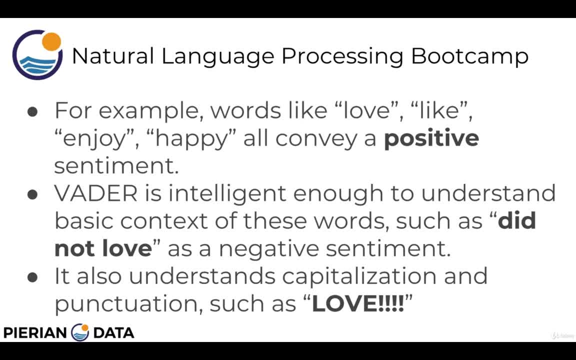 enjoy and happy. Those all convey a positive sentiment. And remember we also talked about emotion And VADER is actually intelligent enough to understand basic context of these words, such as did not love as a negative sentiment. So don't be too concerned about things like having the word. 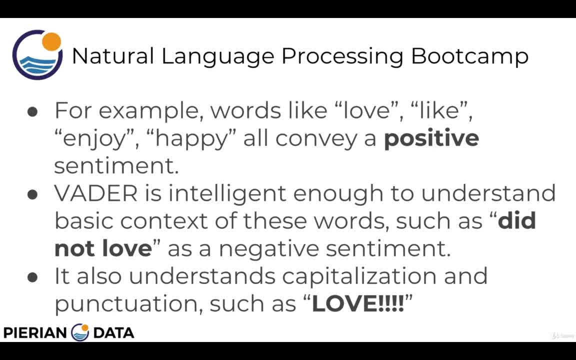 love be completely positive, Because VADER will also take into account the context of the words, because if there's a negative word, such as not preceding a positive word, then you can understand that that whole sentiment is probably negative. So not love or did not like the. 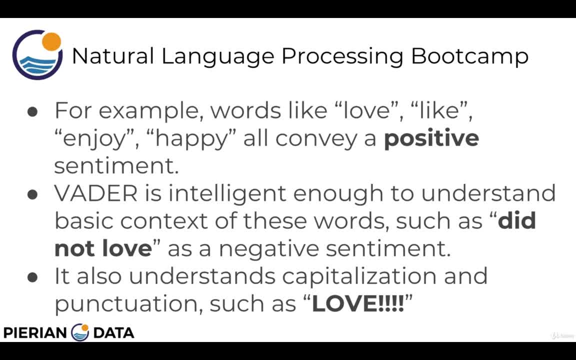 not enjoy. VADER will understand that And it's also going to understand things like capitalization and punctuation. So if you write just a lowercase word, love, that doesn't convey a positive emotion as strongly as love in all caps with a bunch of exclamation marks. So VADER is also smart. 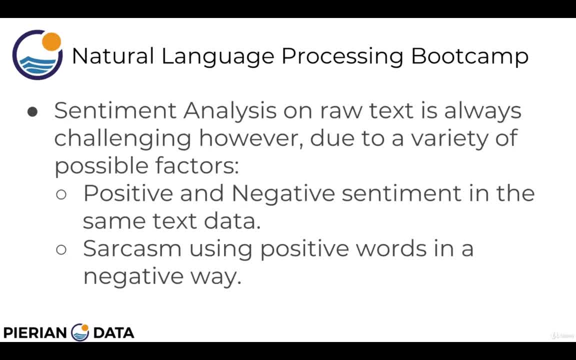 enough to take that into account. Now, sentiment on raw text is always going to be challenging because there's a variety of possible factors, things like positive and negative sentiment- in the same text data. So, for example, if you're reading a movie review, often movie reviews will 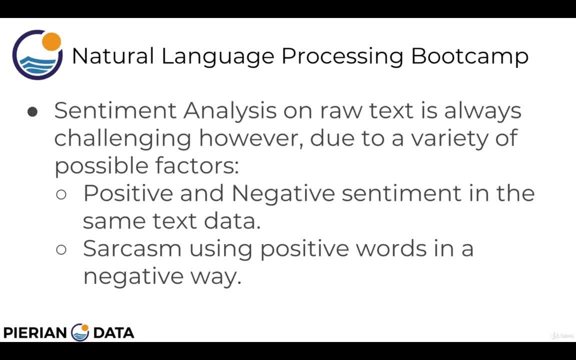 praise actors capabilities. However, maybe they judge the overall screenplay or the script of the movie itself as very poor And, as we know, if you've seen a movie with great actors in it, that isn't a good movie often has to do with the screenplay or the poor script, or just the poor. 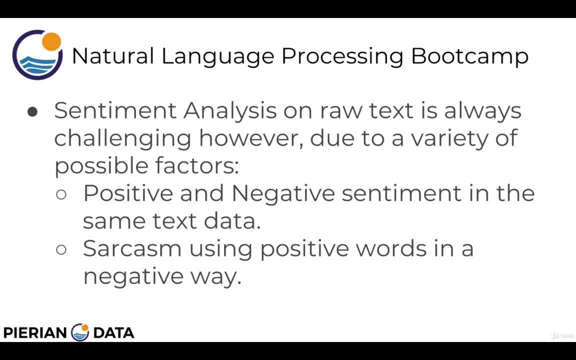 storyline. So a movie review could have a positive things about the actors but then negative things to say, But the overall movie itself? and if there's more positive things about the actors, then VADER is going to say that the overall movie review could be positive, when in fact the true analysis of 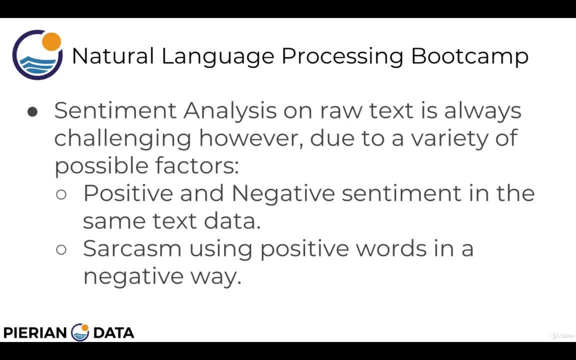 the movie review, when read by human, would be that the overall movie was negative, but the actors were positive in it. Now, another thing that's very difficult to detect is sarcasm. This is pretty much impossible for VADER to detect because you end up using positive words in a negative. 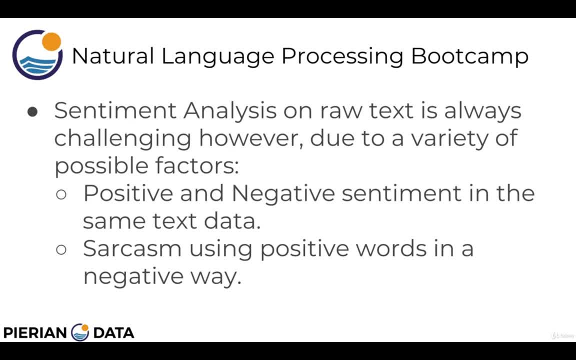 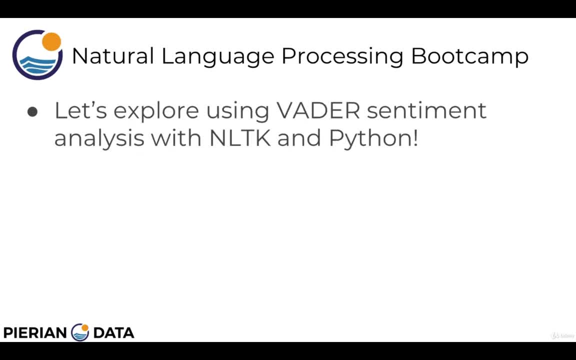 way sarcastically. So keep these two ideas in mind. The sentiment analysis from VADER is definitely not going to be foolproof, So what we're going to do now is explore using VADER sentiment analysis, NLTK and Python. The key thing to keep in mind here is that we're going to be able to apply 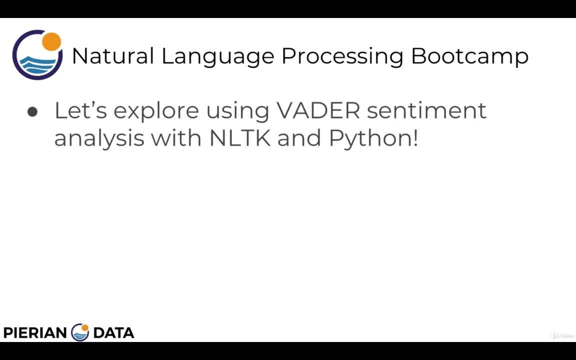 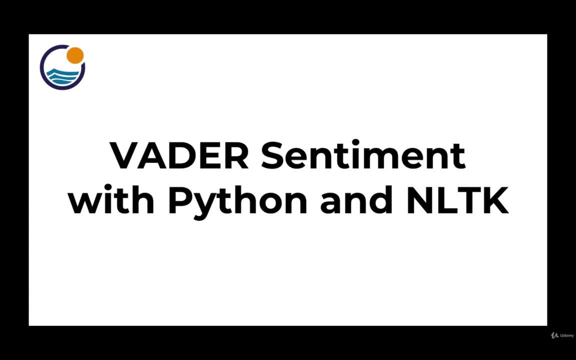 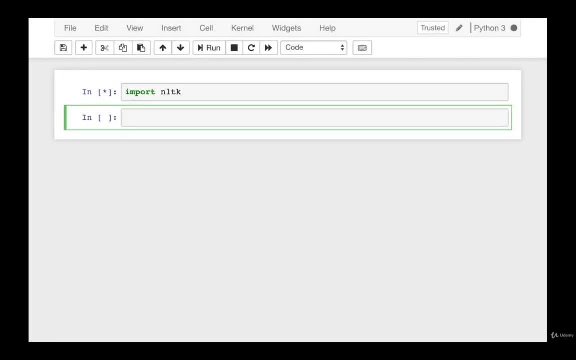 VADER onto any raw text data that we want. Okay, let's get started. I'll see you in the next lecture. Welcome back everyone. In this lecture, we're going to show you how to use VADER sentiment analysis with Python and NLTK. Okay, let's begin by importing NLTK, And then what you need to do is to: 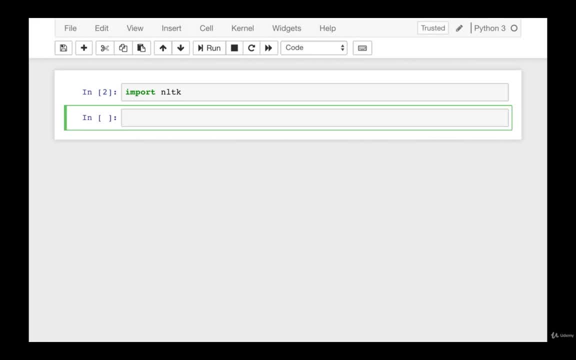 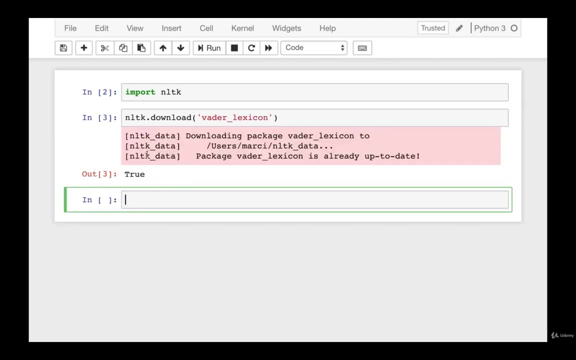 download the VADER lexicon And you only need to do this once. So we'll say NLTK, download And then pass in VADER underscore lexicon. Go ahead and run that And then, if you've already downloaded it, it should be almost instantaneous. If not, it may take a little bit of time to download the data from. 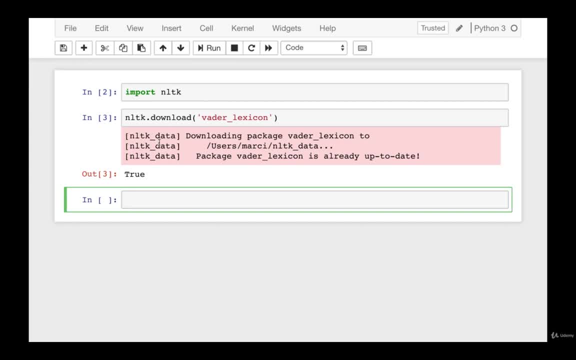 the internet. Make sure you check your firewall and make sure that's not blocking your download. So once you've downloaded the VADER lexicon you should be able to import it And then you're going to start using from NLTK dot sentiment dot, VADER import and then it's sentiment intensity. 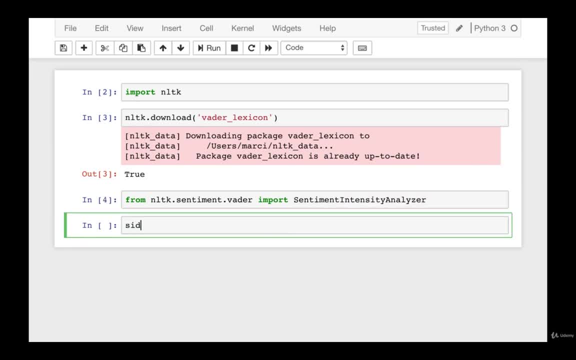 analyzer And then create an instance of it. we call it SID. And what VADER sentiment intensity analyzer does is it simply takes in a string and returns a dictionary of scores in four categories: negative, neutral, positive and then a compound score. 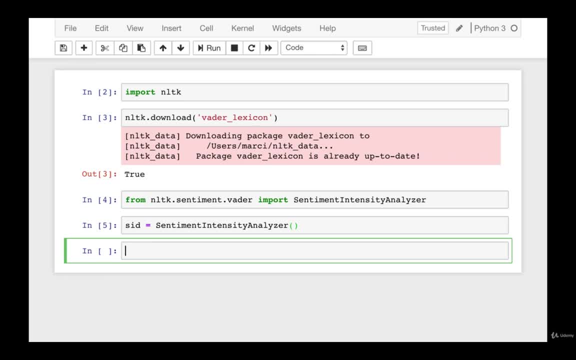 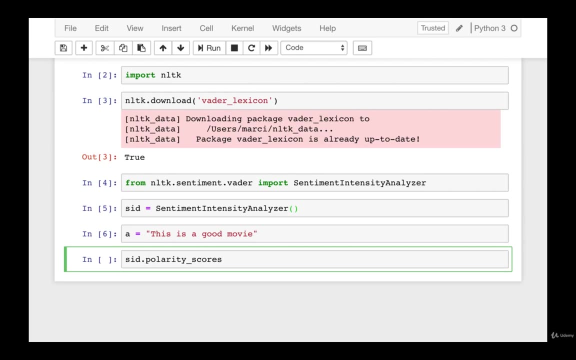 which is computed by normalizing the negative, neutral and positive scores. So let's create a really simple string. we will say this is a good movie, And then we'll say SID, dot, and off of this we will call polarity, underscore scores and then pass in the string And you get back this: 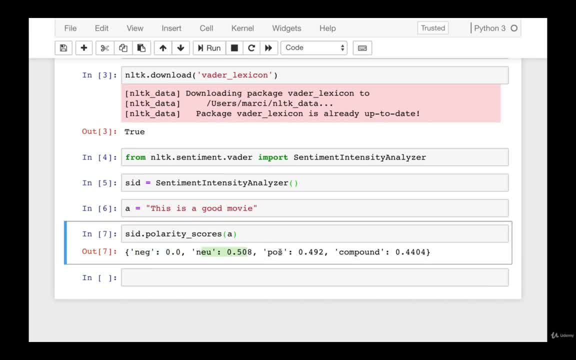 dictionary which has some negative value, a neutral value, a positive value and then a compound value which is essentially normalizing these three values here. So, as we expect, there is no negative value, since it's this is a good movie, It has some neutral. 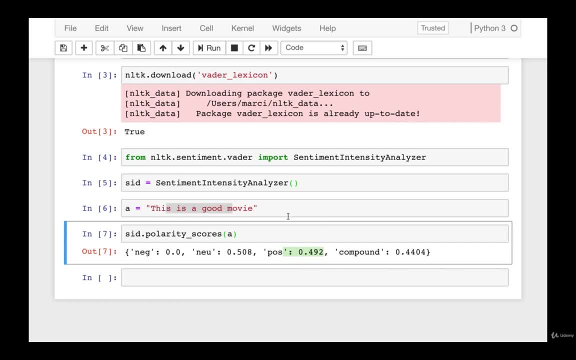 words or tones in it. And then it has also some positive tones And the max value for any of these is 1.0.. So now let's try a more complicated string. We'll say: this was the best comma, most awesome movie. And then we're going to capitalize ever made and have three exclamation. points. And, as we previously mentioned, VADER is the best movie ever made. And then we're going to capitalize ever made and have three exclamation points. And, as we previously mentioned, VADER is the best movie ever made. And then we're going to capitalize ever made and have three. 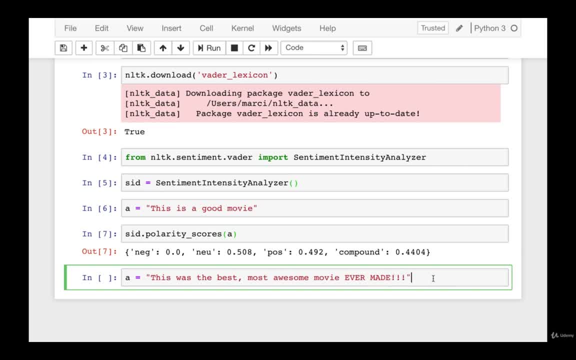 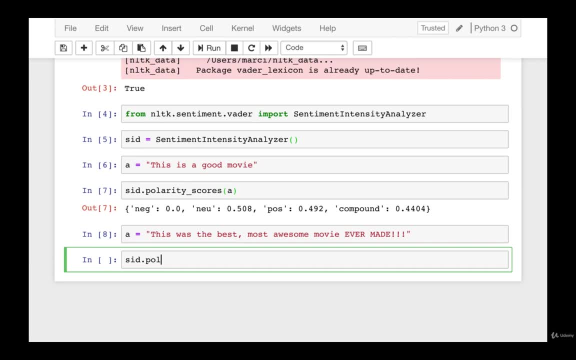 exclamation points. And then we're going to capitalize ever made and have three exclamation points. And then we're going to capitalize ever made and have three exclamation points. So we'll go ahead and run that And then again call s ID polarity scores. oops, make sure we spell that. 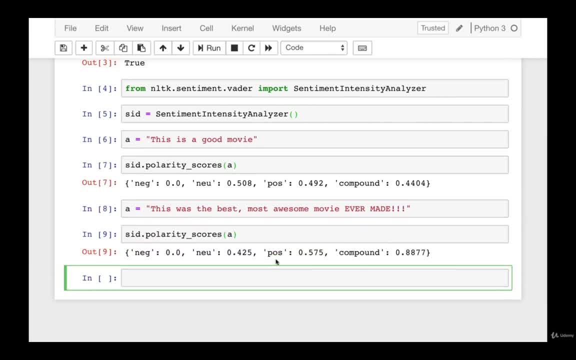 right Pass in the string And here we can see it's again more positive than the previous one, And we can see here that the compound score is much more positive because neutral also dropped. Finally, let's go ahead and have a very negative string, So we'll say this was the worst movie. 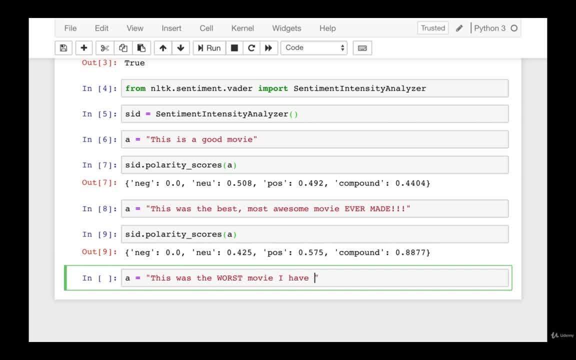 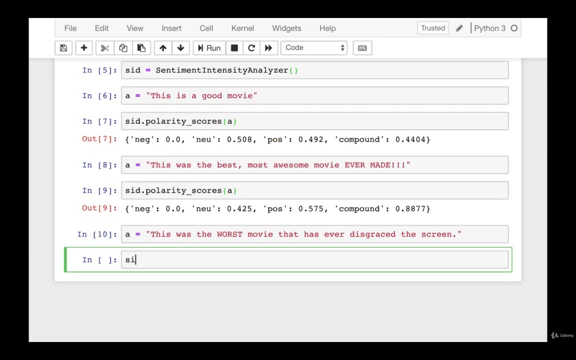 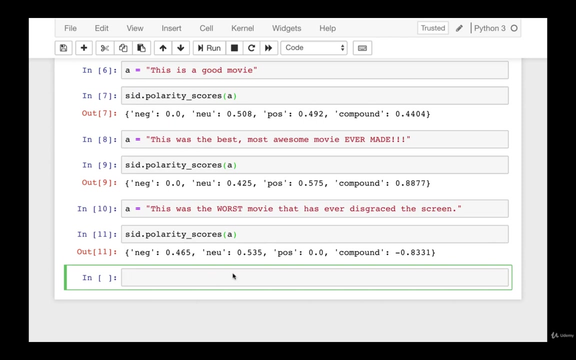 I have ever, or that has ever, disgraced seeing. let's say that has ever disgraced, disgraced the screen. Okay, so quite a negative review. Let's see if the VADER picks it up. We'll say: s ID polarity scores pass an A, And here we can see that now there is no positive. 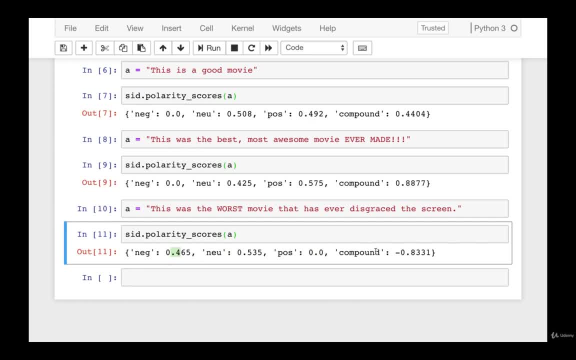 it's just neutral and negative. And so what happens is the compound score then becomes, then becomes negative. So we can see here: a compound score of zero would be completely neutral. A compound score above zero indicates some sort of positive score, And then a compound 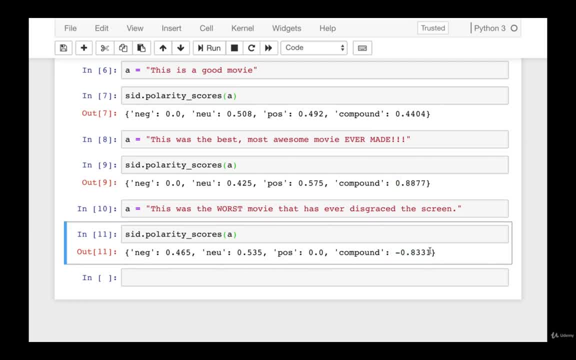 score below zero indicates some sort of negative score. So now what we're going to do is show you how you can use VADER to analyze Amazon reviews. So in our text files folder we have an Amazon reviewstsv file. I went ahead and moved it to the same location as my notebook here And we're 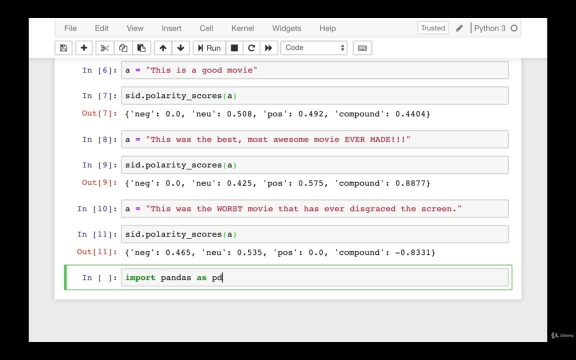 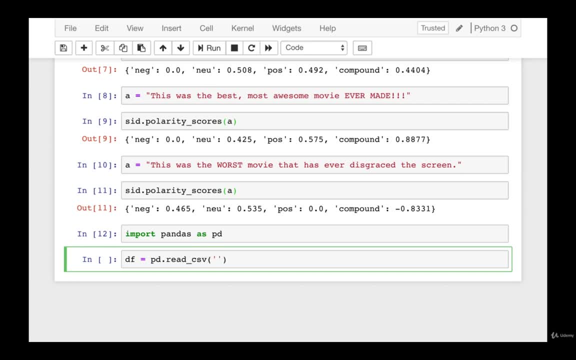 going to read it in And then we're going to go ahead and paste it in here, And then we're going to paste it in using pandas. we'll say: import pandas as PD, And then we'll say DF is equal to PD. read CSV, And I already moved the file here, So it's simply called Amazon reviewstsv. It's. 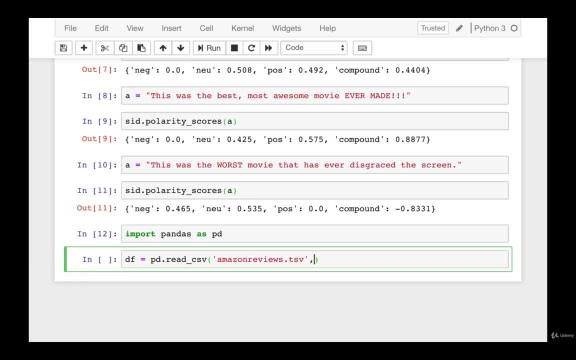 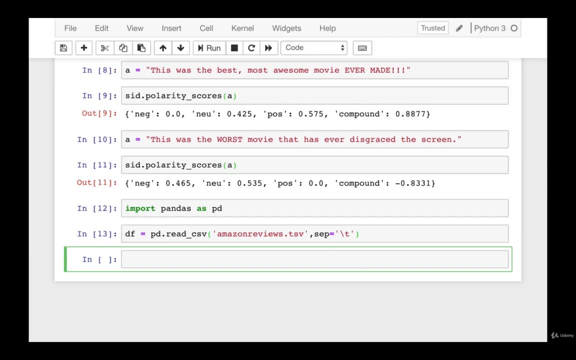 again located under text files folder And it's tab separated. So you need to also indicate that the separator is backslash T for tab separation. Once you read that in, you should be able to view it by simply calling the head of that data frame. And essentially what we have here. 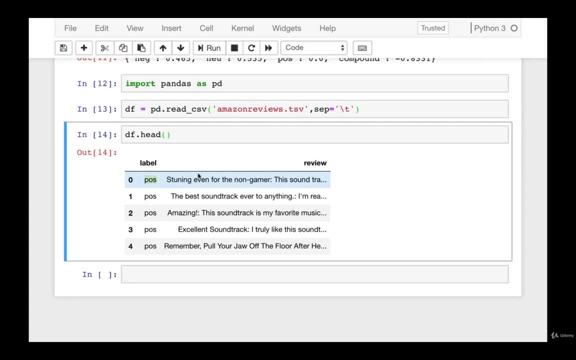 our labels. they see their POS for positive or energy for negative, And then we have the actual text of the review. So if we wanted to get an idea of how many positive versus negative labels we want we have, we can say DF, pass in the label column and then simply call value underscore. 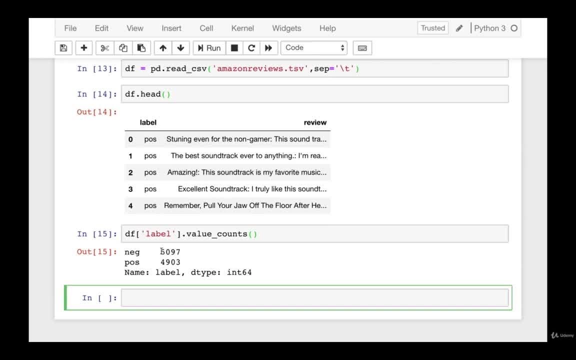 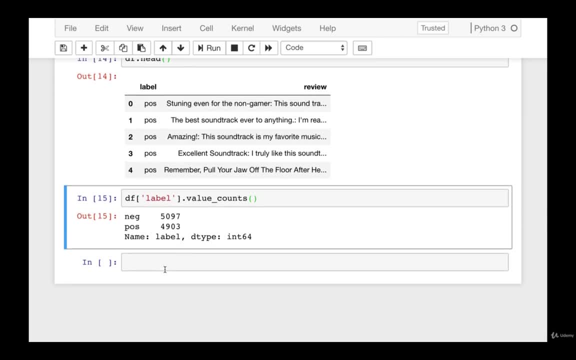 counts, And we can see here we have slightly more negative reviews than positive reviews, But overall it looks like we have around 10,000 reviews. So what we're going to do now is do a little bit of cleaning of the database And then we're going to go ahead and do a little bit of 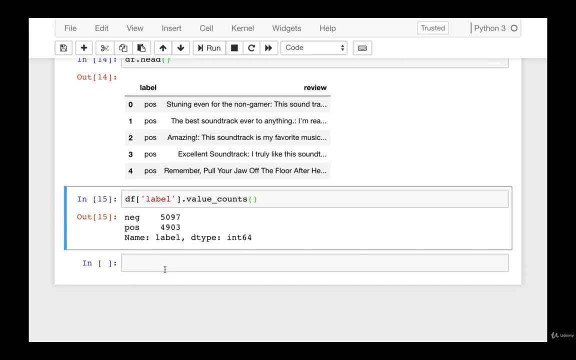 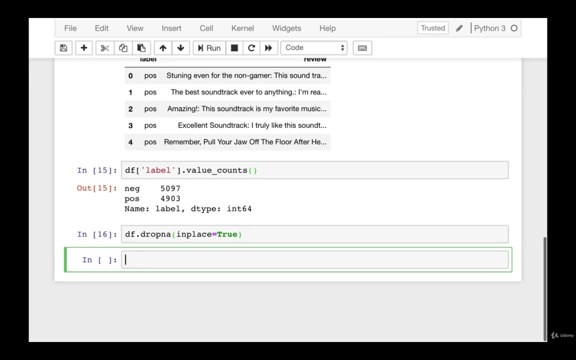 cleaning of the data just to double check that we have no empty records, And then we're going to run a first review through Vader. So, quite simply, what we're going to do here is simply say DF, dot, drop na. And we'll say: in place is equal to true. that's going to drop anything that's missing And 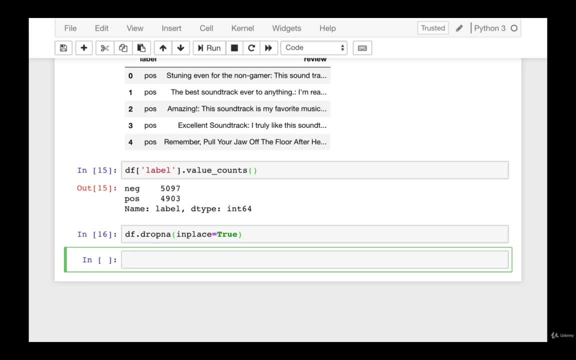 then what we're going to do is drop anything that has a empty whitespace value. Now for your data sets. depending on where you get them, you may or may not have this, but it's always a good idea. I'm just saying for index, for label and for review. So those are kind of placeholders there. 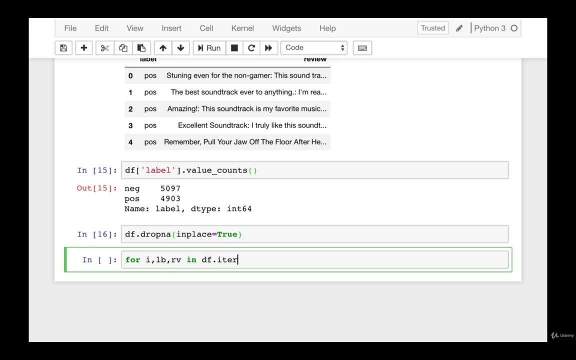 and DF dot, and then I'm going to call iter tuples. So essentially here everything is just going to be returned as a tuple where I have the index, the label and then the review text. So for I label and review, I'm going to say if the type of the review is equal to the string. 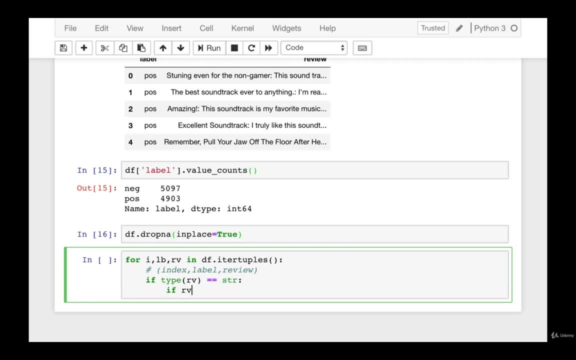 then I'm going to check that the review is space, essentially checking whether or not it's a space there- And if it's true, I'm going to take a list of blanks, which let's go ahead and define it. We'll say blanks, And we've already seen this kind of thing before, But we'll simply say blanks. 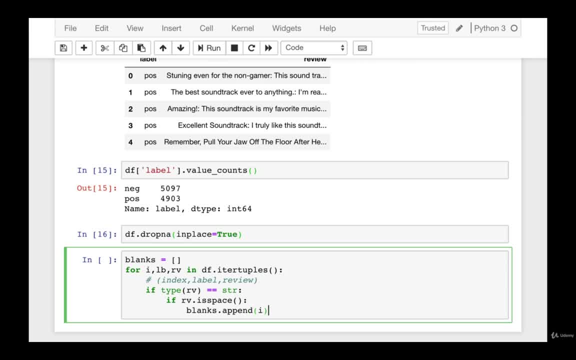 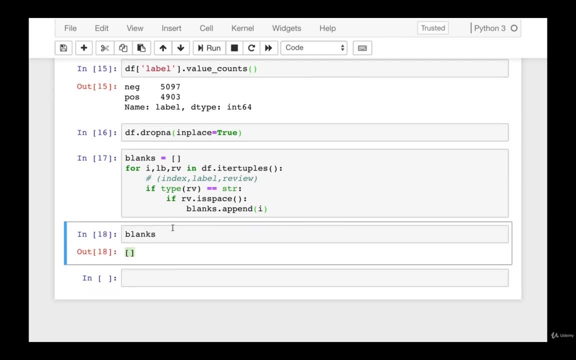 append and then we'll plan that index position. So if we run this, let's go ahead and check on blanks. See if we had any blanks. It looks like we didn't. this list is empty, So we don't need to drop anything. But if we did have some index positions that were blanks, 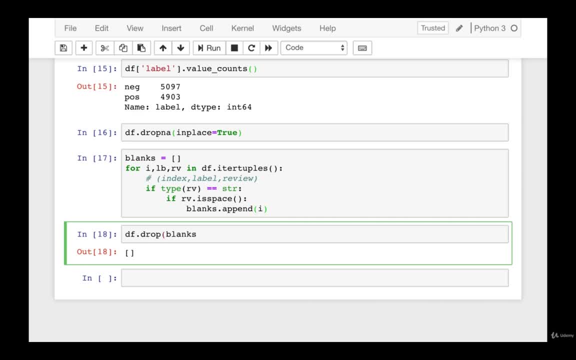 we simply needed to say: DF, drop blanks, And then we could say: in place is equal to true. But again, since we don't have any, we don't actually need to run that line. So now what we're going to do. 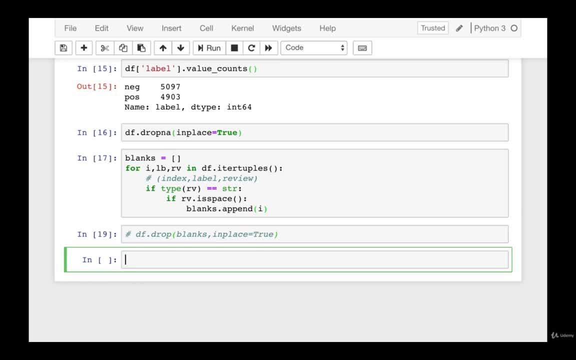 is: continue on and run a first review through Vader. So we'll say SID, call polarity scores and we're going to just run the first review on it. So we'll say DF, dot and we'll call ILOC zero and then call that particular review. So all I'm doing is, if we 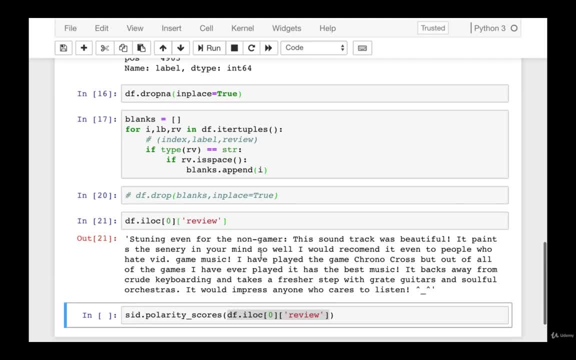 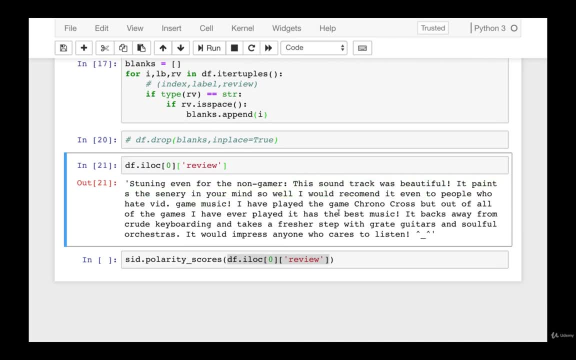 were to check out this one line here. that's essentially just grabbing the text of the first review. So we can see here it's quite positive. the soundtrack was beautiful, game music, exclamation points, best music, etc. So let's check out the polarity score here And then we 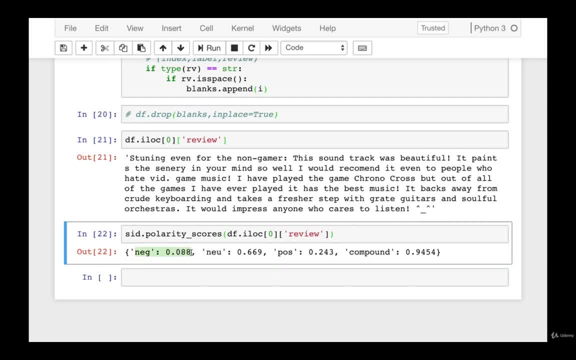 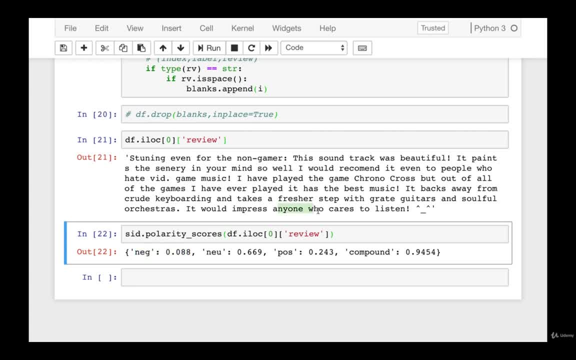 small phrases that get confusing for Vader things like anyone who cares to listen- maybe kind of negative in a slight sense, but it's actually a very small negativity. In fact, most of it is neutral or slightly positive, which means the compound score is. 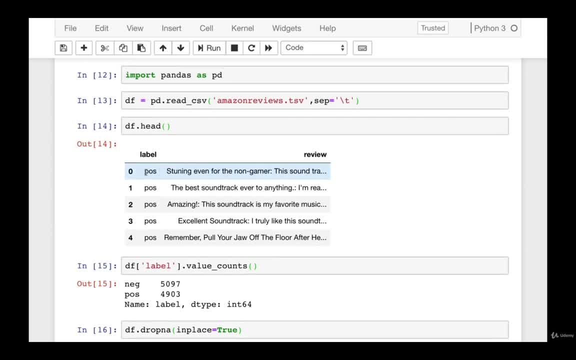 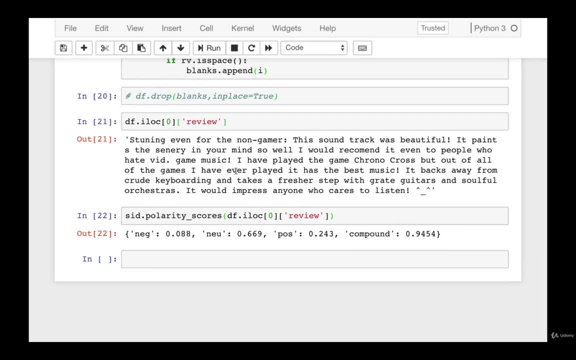 extremely positive which, if we take a look at that first label, was positive. So the first few reviews are positive. So it looks like Vader is actually able to select that. So now let's go ahead and add scores and labels to the data frame. So we're going to say DF. 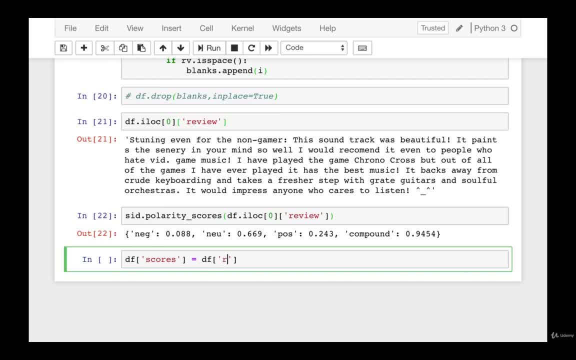 scores is equal to DF review. And then we're going to call an apply method in order to essentially apply SID polarity scores to every single review in our data frame. So we'll say lambda, take that review and then apply SID polarity scores to that particular review. 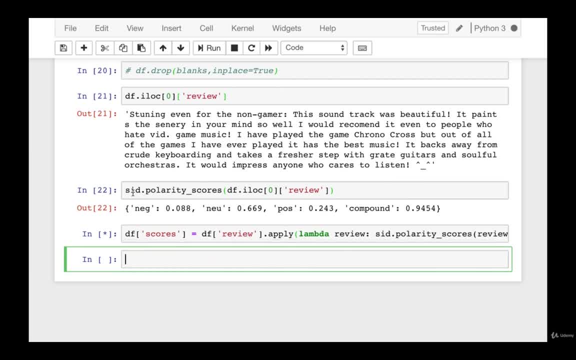 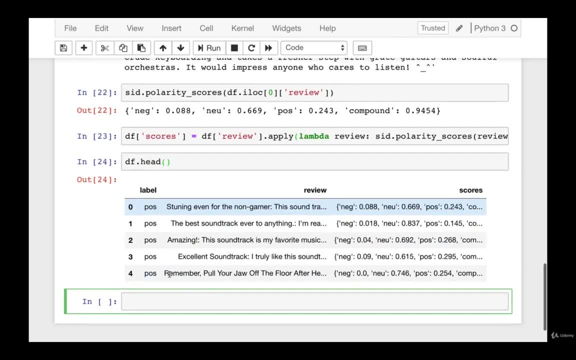 So we run that And this may take a little bit of time because it is running this whole polarity scores function on every single review, But once you have that you can go ahead and check out the head of the data frame And then you'll get back a new column scores that contains this dictionary And often 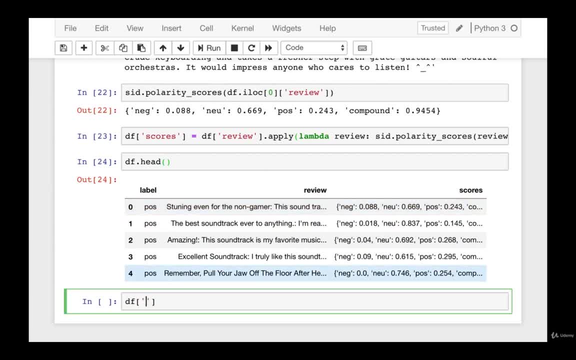 you really just want to deal with the compound score. So let's go ahead and create a new compound column. we'll say DF compound, And then we'll set that equal to DF scores And similar idea. here we're simply going to apply a lambda And we're going to pass in that dictionary and then just 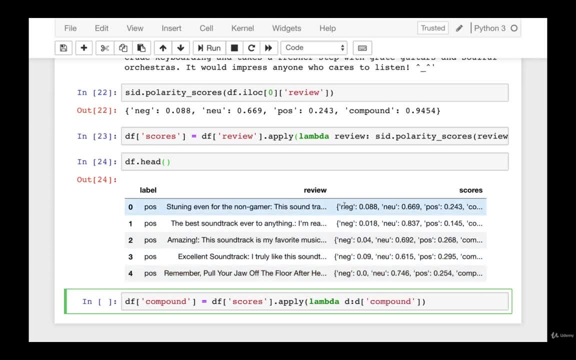 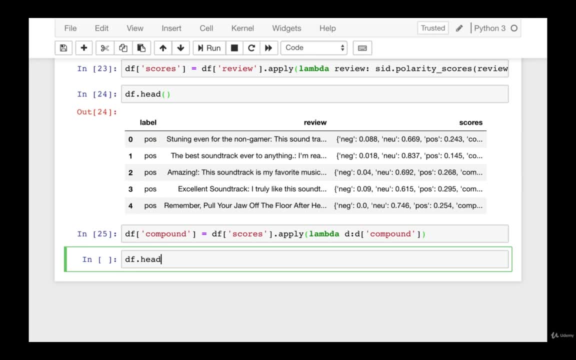 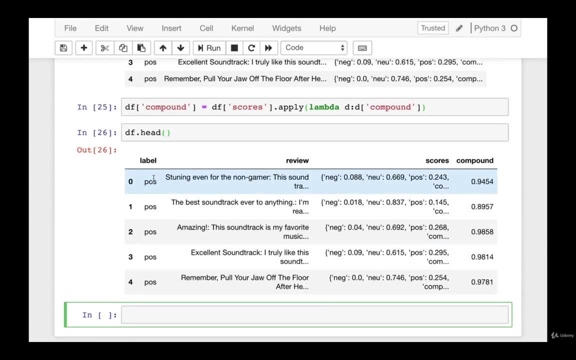 grab compound off of that dictionary. So every item in scores is a dictionary source is just reading the score for compound. So we'll go ahead and run that. That's going to be much faster since the dictionary is just existing there, And then we can get the compound score. So notice these first five labels. they're all positive. 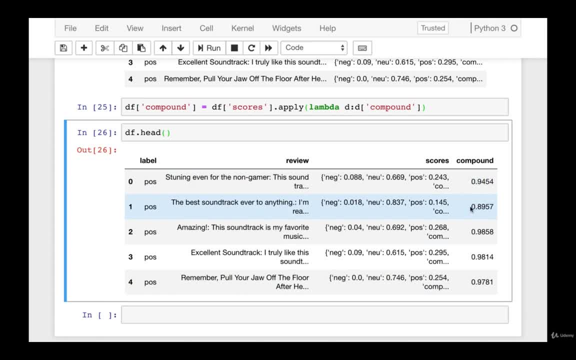 and it looks like the compound score is also all positive. So let's go ahead and, based off this compound score, do a little bit of logic and say if it's greater than zero, then it's positive, If it's less than zero, it's negative. And then we'll compare these compound scores. 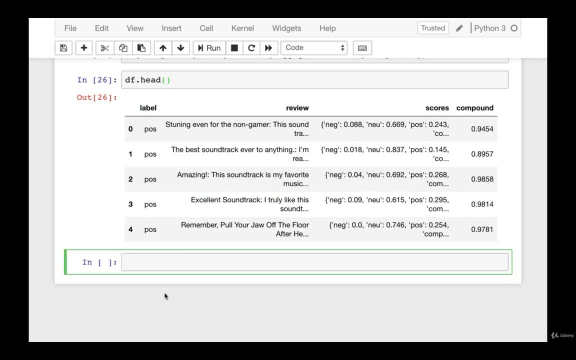 to the true labels that we already know. So we're going to say one last column of our creation comp score and say it's equal to DF compound And we're going to apply essentially a little bit of logic here. we'll take in that score. 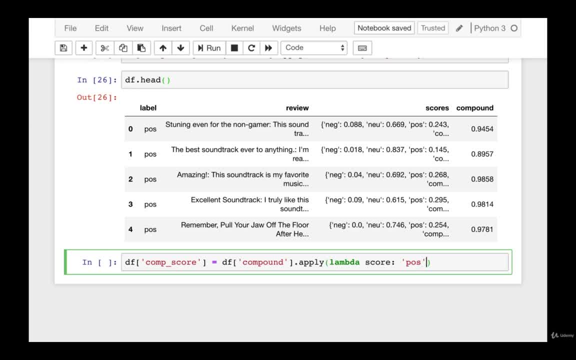 And we'll say: return back the string POS for positive if the score is greater than or equal to zero. else return the string negative, essentially changing the score into a string that matches our current label. So if we run this and then again, 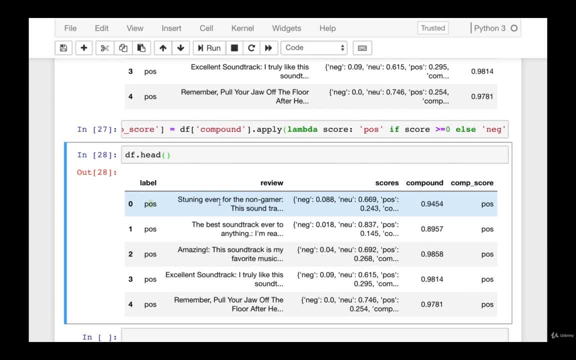 check out the head of our data frame. Now we have a label, the review, the full scores dictionary, the compound off of that scores dictionary and our converted compound to a score or a label POS. So it looks like we're matching up on the first five, But let's go ahead and have an overall. 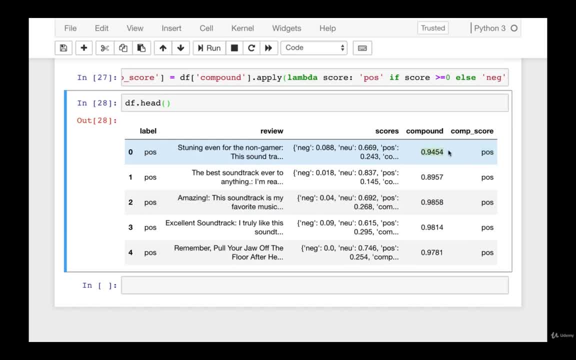 report on the accuracy comparing the vader compound score labels to the manual labels from this data set. And we can do that simply by saying: from sklearnmetrics, import, and we'll do an accuracy score, a classification report as well as a confusion matrix. So we've already seen quite 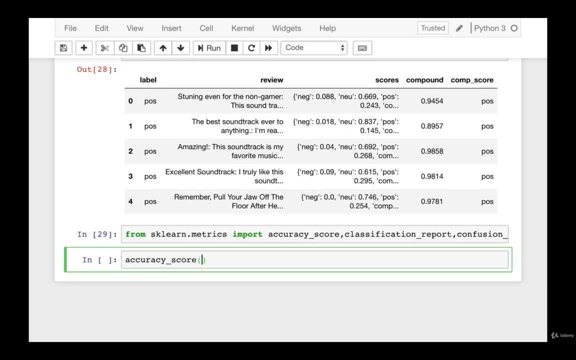 a few of these already. let's first just get the accuracy score, And we can do that by simply saying df of label. So that's the correct value compared to df comp score. So essentially we're comparing. how well did vader perform against what was manually labeled? So this first label was: 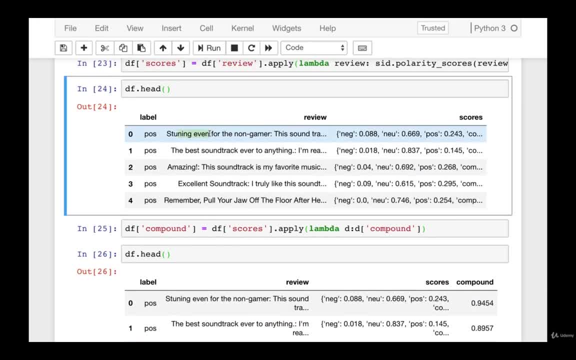 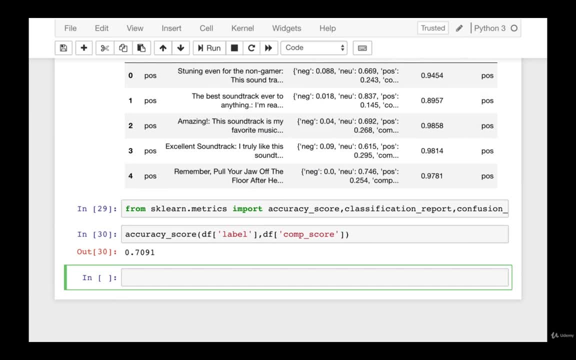 manually labeled. essentially, a person read these reviews and decided whether or not they are positive or negative. So if we run the accuracy score, we get an accuracy of 0.7.. If we were to randomly choose positives and negatives, we'd be probably getting an accuracy. 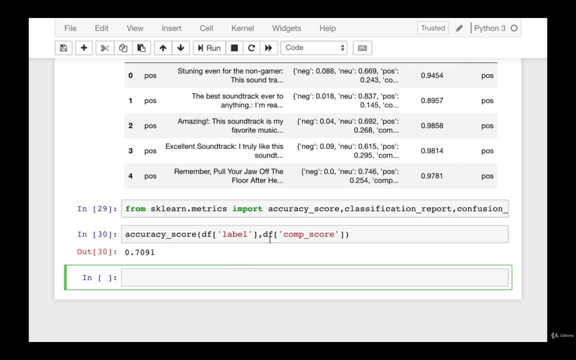 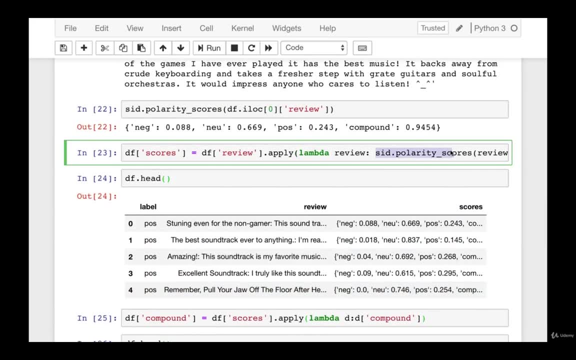 of around 0.5.. So we can already see we're doing better than random guessing, which is quite good, given the fact that we're essentially just running one line of code up here of SID polarity scores. So it's definitely not bad, considering how simple it is to run this process. Let's go ahead and. 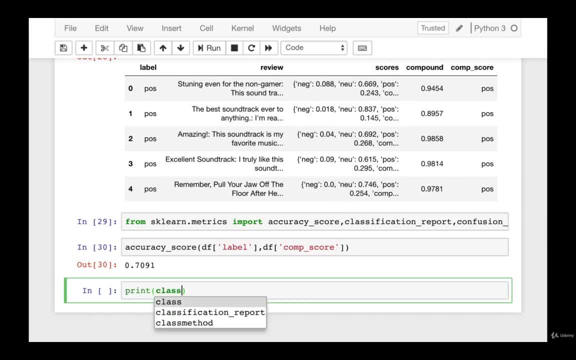 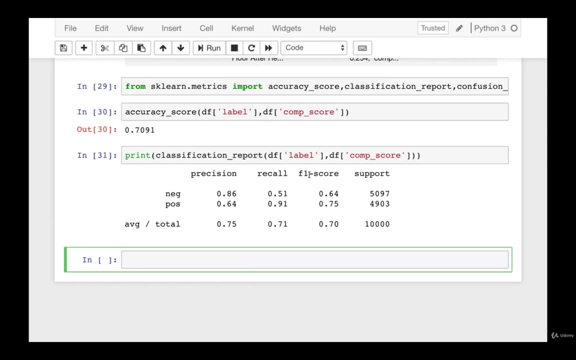 print the classification report. We'll say print classification report And just like before, we'll pass in the true label that we know and then our calculated comp score. So we'll run this and then we can see our precision recall an F1 score And we can also compare it to versus. 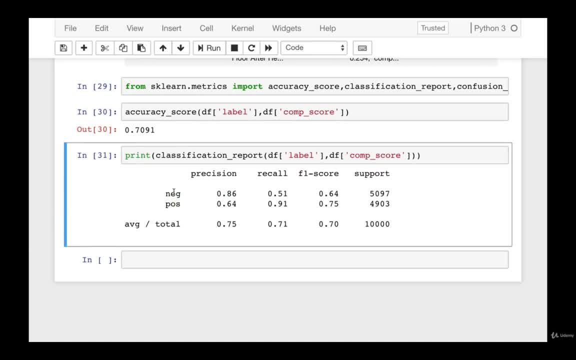 negative versus positive. So it looks like the Vader has a little bit of trouble with negative reviews versus positive reviews And if you take a look at some of these Amazon reviews, some of these strings and some of the text is sometimes a bit hard to read. So we're going to go ahead and 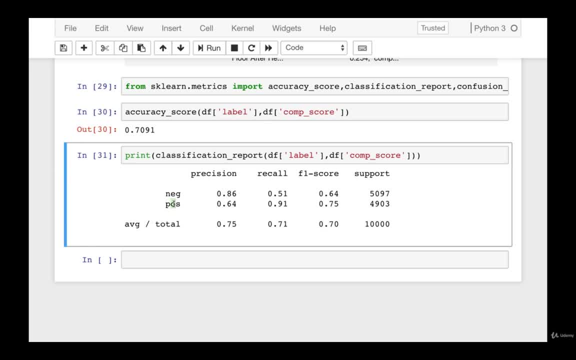 hard to read And sometimes it's also sarcastic, which means it's really hard to detect. So sarcasm is almost impossible to detect for something like Vader. And then finally let's print out a confusion matrix, So say confusion matrix and then DF label and pass in what Vader.